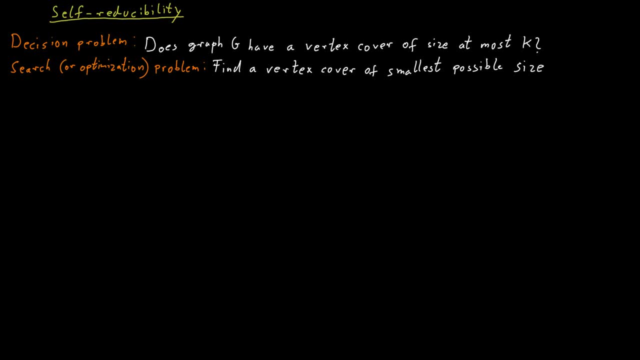 but for cook reductions, X doesn't need to be a decision problem. So what we will do is we will define something called a polynomial time cook reduction. A polynomial time cook reduction is just like a cook reduction, but we require that the oracle machine runs in polynomial time. 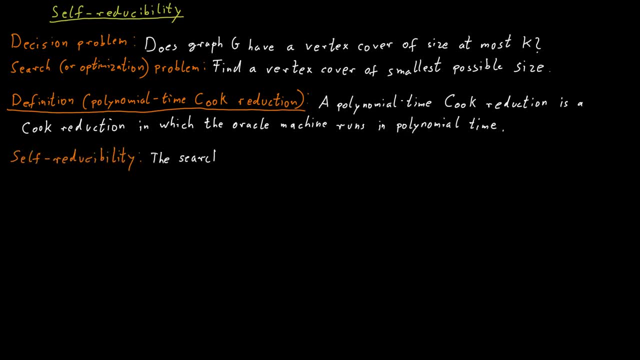 Now. self-reducibility means that the search version of a problem, polynomial time cook, reduces to the decision version of the problem, And the problem is just going to be done there, As only then can Ar数 be��j ΚrUĘΙ oÉ incubated. 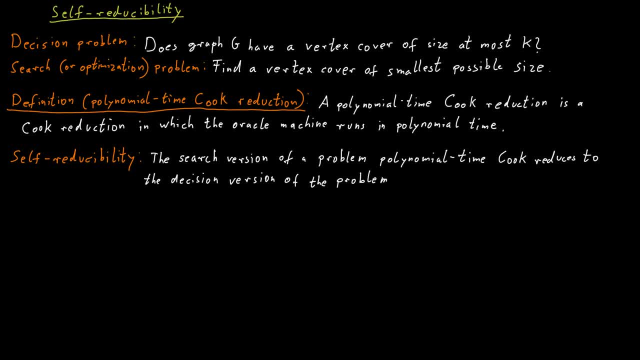 And this holds for all the problems we discussed. And what this means is that if we can solve the decision version of the problem efficiently, we can also solve the search or optimization version of the problem. We just take the search version of the problem and then apply the cook reduction and 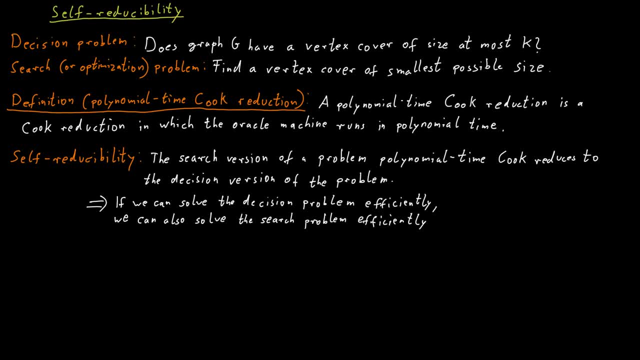 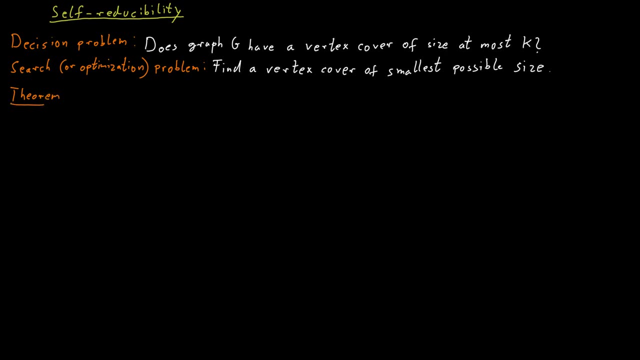 use the algorithm that we have that is efficient for the decision version, as this subprocedure that the oracle calls. So really, the search problems are not really harder than the decision problems. Let's look at a specific example. Let's take vertex cover. 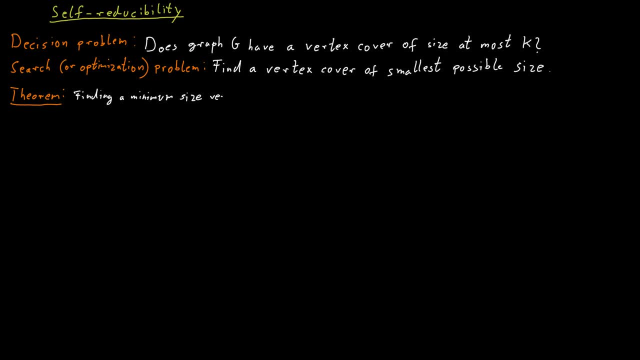 I claim that if I have an algorithm that can decide whether a vertex cover of size at most k exists, I can use this to build an algorithm that finds the minimum cardinality vertex cover of a graph and does so efficiently. So the first step is to find out. 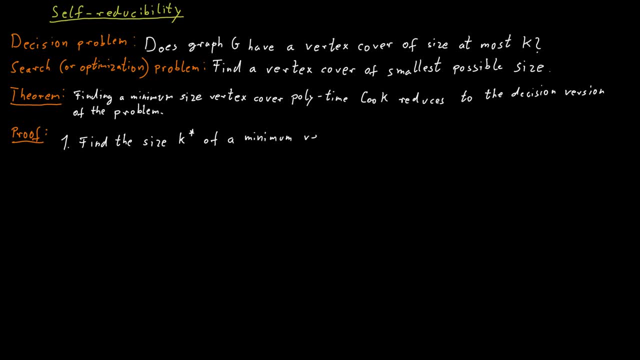 what the size of the minimum vertex cover is. What is the cardinality of the minimum vertex cover? For this we just try all different values for k. So we just ask: is there a vertex cover of size 0?? If the answer is no, 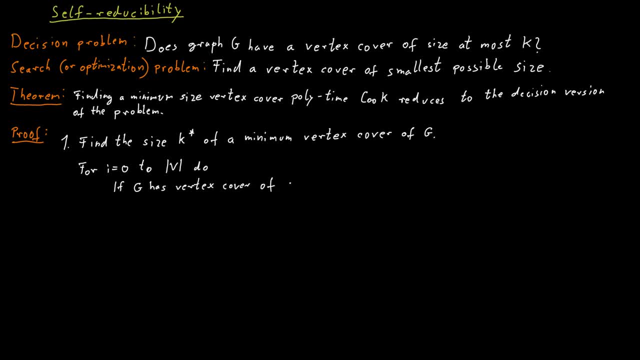 we just ask, okay, is there one of size 1?? If the answer is no, we just say, well, is there one of size 2 then? And we keep going up until the answer is yes. So then we know what the minimum size. 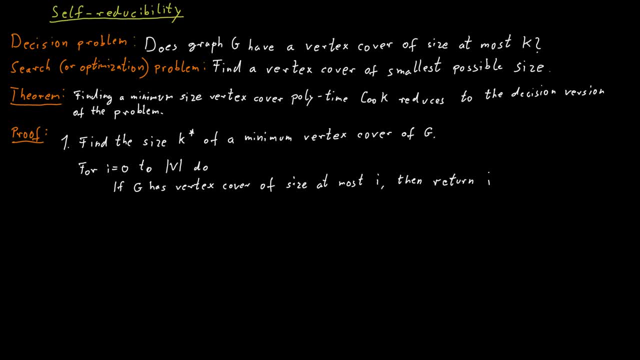 of a vertex cover is, If you're very clever you might say this is very inefficient. What we really should do is we should do binary search here, So we should kind of try to narrow down the value more quickly. But both methods work in the sense. 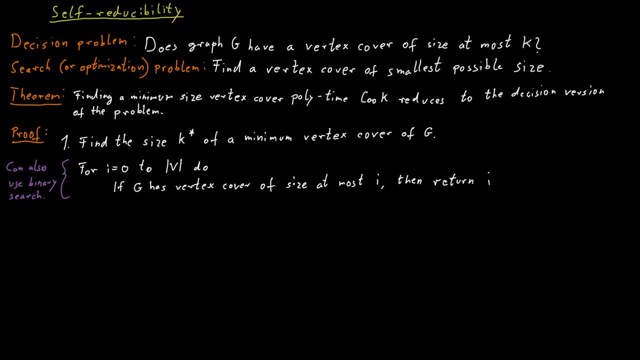 that both methods will be polynomial, Because if I do this linear search, how many times will I ask the oracle? at most, Well, I start at 0, and then I know there's a vertex cover of size n, when n is the number of vertices. 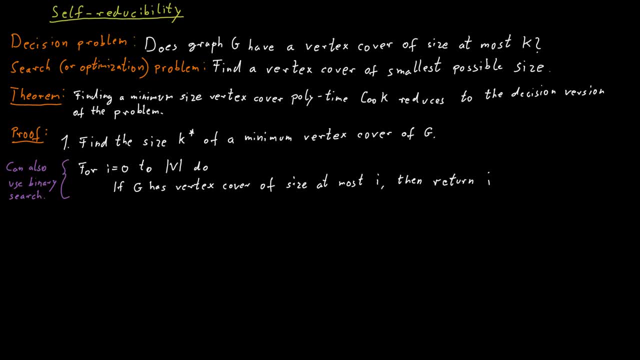 in the graph. So I will only call the oracle size of v many times. So now we know how large the minimum vertex cover should be. Let's call the size of the minimum vertex cover k star. Here's how we find such a vertex cover. 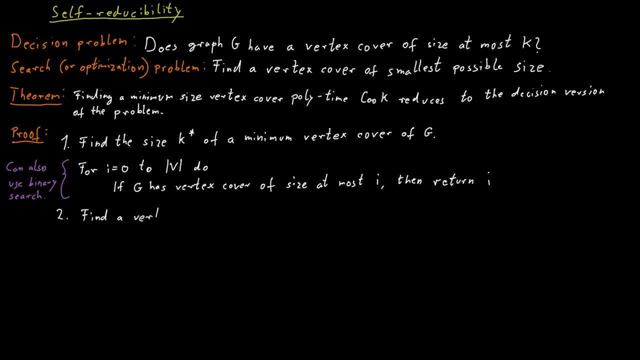 We take the graph and we look for a vertex v, such that if we remove the vertex v from the graph then the remaining graph has a vertex cover of size at most k star minus 1.. And we can check for each vertex v whether the remaining graph 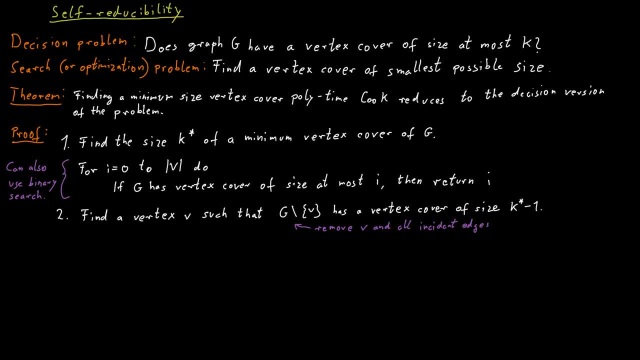 would have a vertex cover of size at most k star minus 1, using our oracle, using access to this algorithm for the decision problem. So we just go through all the vertices of the graph one by one, We check each one, remove it from the graph. 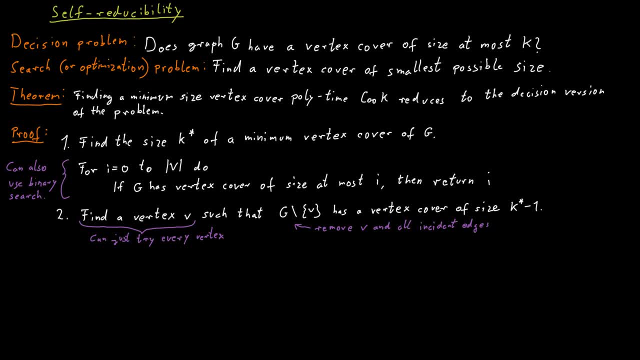 see if the remaining graph has a vertex cover. If yes, we found a vertex v that works. If no, we move on to the next vertex. Now, important here is that there exists such a vertex for sure, So eventually we will find one.